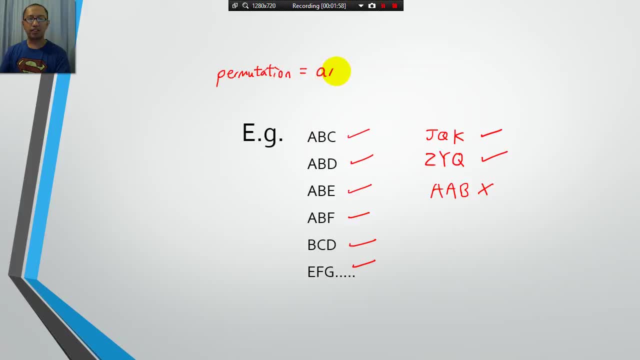 the same word as arrangements. So when the question says how many arrangements are there, it's the same thing as saying how many permutations are there. Permutation means that the order is important. Now, what that means is, for example, ABC is different to BCA. 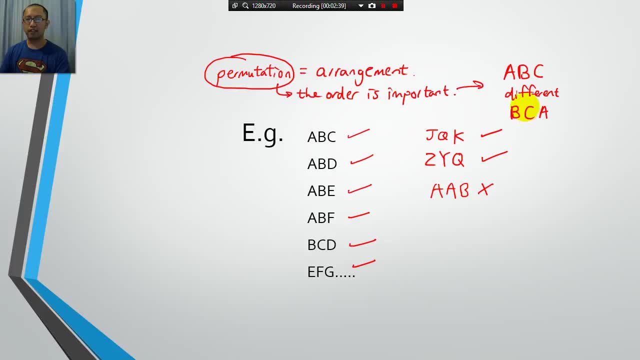 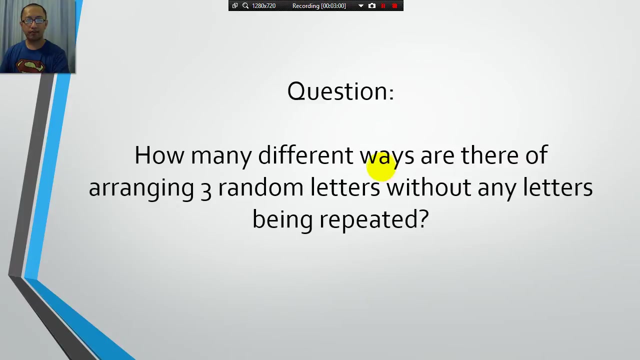 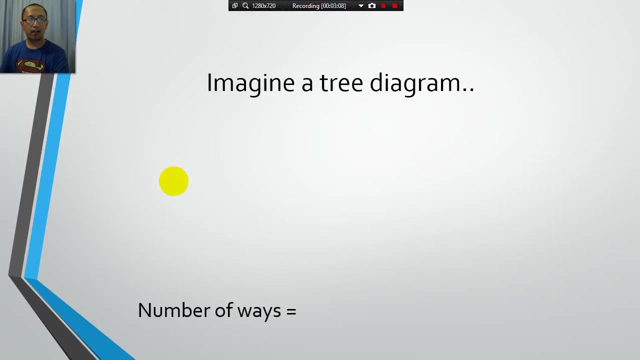 Even though they contain the same letters, but because we ordered them differently, they count as two arrangements, Two permutations, Or in other words, two ways of arranging. So how many ways are there of arranging three random letters? How many permutations are there? Now we're going to solve the problem by drawing a tree diagram, because it's going to be a 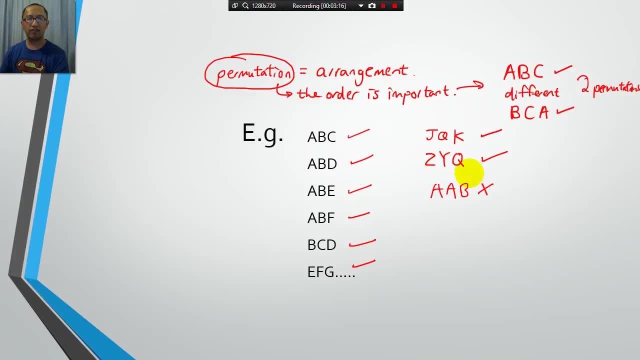 bit hard for you to write out all the different combinations. It'll take you forever. So if you draw a tree, however, Then what happens is the first letter. you have 26 options. You can start with A, B, C. okay, 26 options. 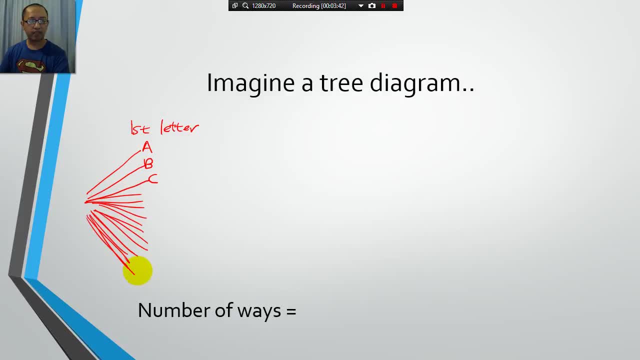 But we're not going to write all of them out. But anyway, we have Z in the end And there's 26 options. And then let's say we Select any of these. It doesn't matter which one you select, because once you have selected it, 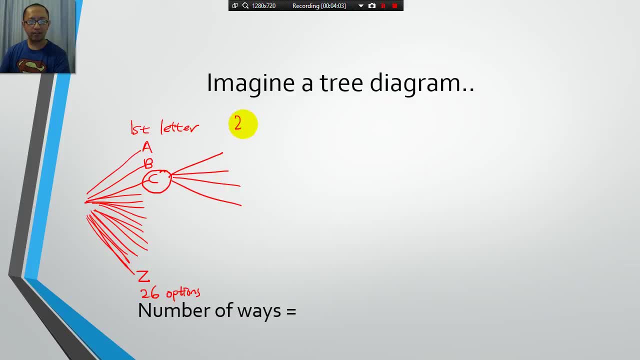 When you pick the second letter. When you pick the second letter, You only have 25 options remaining, Because you can start with A and then go down to B, But you can't pick C again because we don't want repetition In our original question. it says: 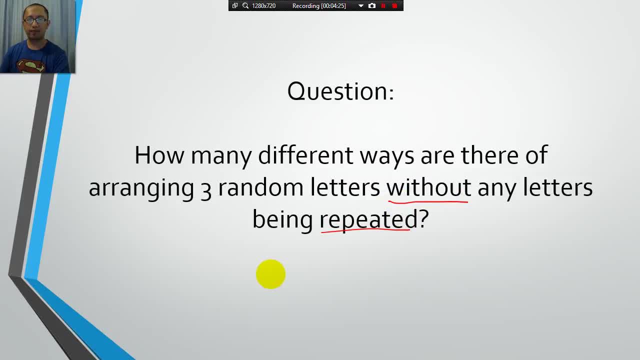 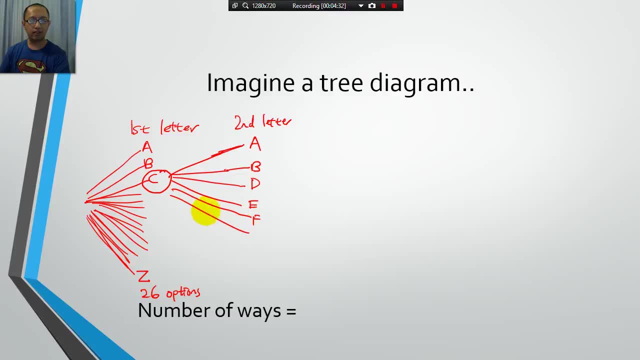 Without repetition. So therefore we can't have C again. We go to D, E, F, G, all the way to Z. So therefore we have 25 options or 25 ways. And then the third letter. Let's say we pick C, A. 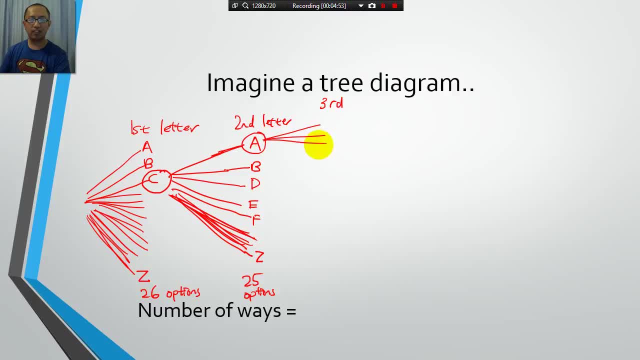 And how many options can I extend From this node? I can't use A again, but I can use B. I can't use C again, but I can use D, E, F, G, All the way to Z. So then I only have 24 options. 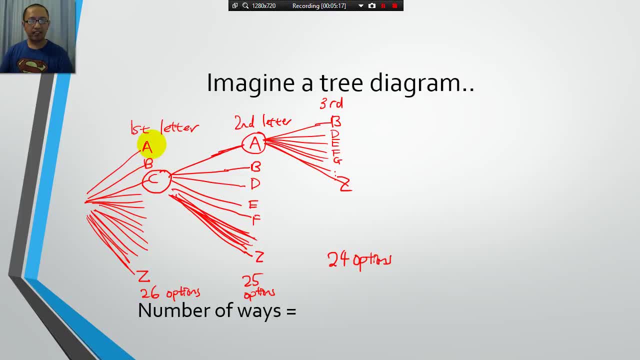 Okay, And basically Every single Option From the beginning, After the first letter, You're going to have 25.. And then Every single Node, from the second letter to the third letter, You're going to have 24.. 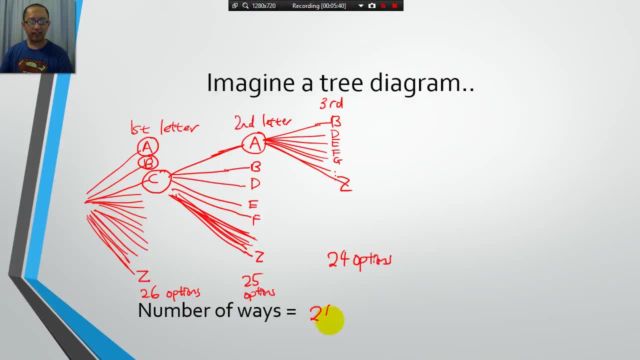 So, therefore, the number of ways is 26 times 25 times 24.. And if you put that in the calculator, The answer is going to be 15,600 ways. 15,600 ways of writing out three letters from the alphabet. 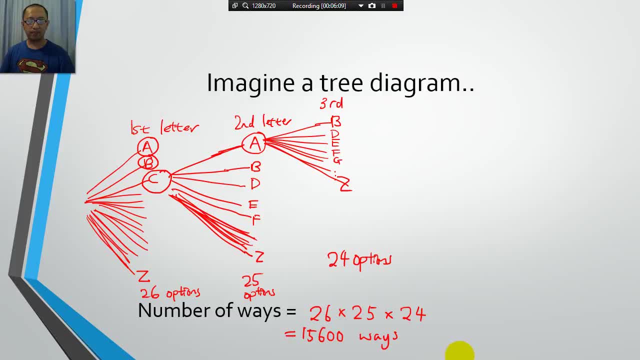 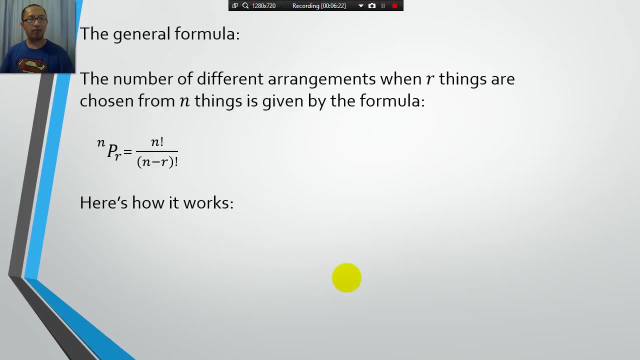 Where each way has a different arrangement, Different order And no letters are repeated. Okay, so it's all good doing it out of a tree diagram, But we want a faster way. We don't have to draw a tree every single time. So the general formula for doing this: 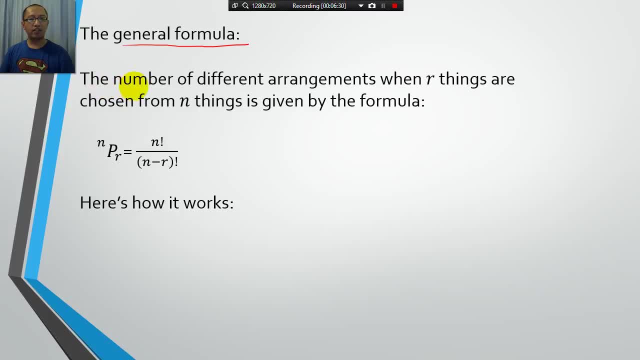 The general formula is: When you are, The number of arrangements when r things are chosen from n things, Is given by this formula. So that's essentially what we're doing: We're picking r things Out of n things. We're picking. 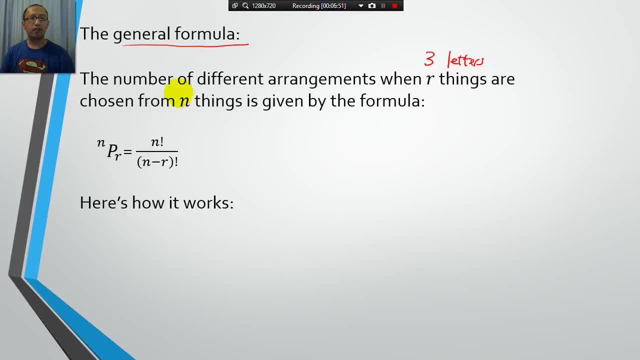 Three letters From 26 letters, Right, and how many different arrangements can we have? So this is the formula: NPR equals n factorial over bracket, n minus r factorial Now, Because n is 26.. We're picking from 26 letters. 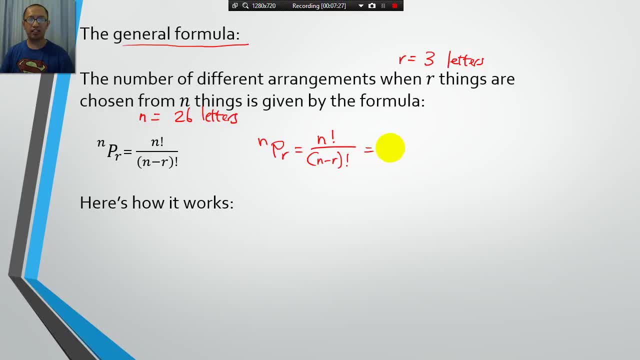 R is 3.. We have to pick 3 letters out of 26.. So you put 26 where n is in the formula And you put 3 where r is in the formula, And now we have to Write the factorials out to simplify it. 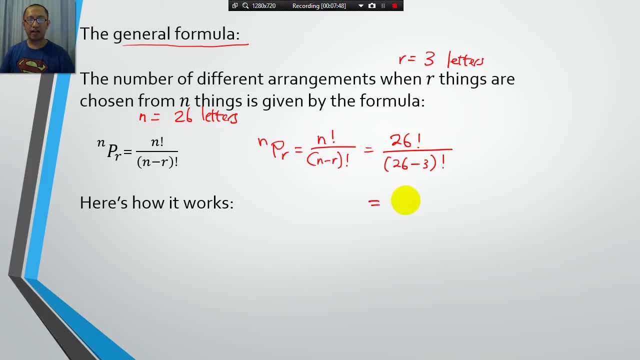 And now we have to Eyedpler. But you could Do it in the calculator. You could just go 26 factorial Over 23 factorial And it will give you the answer In a calculator. But Just so that we show you why it's the same. 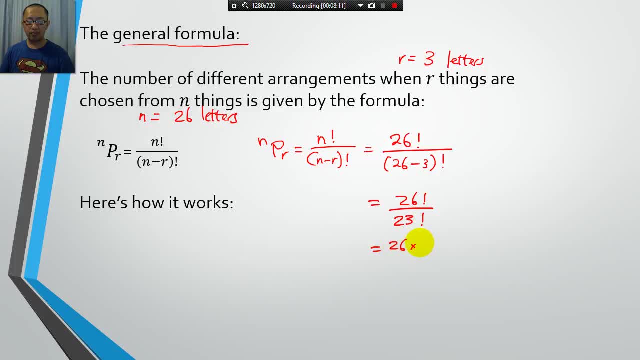 Um. 26 factorial is 26 times 25 times 24.. Times 23. And so on, 1 times 1.. 23 factorial is 23 times 22 times 21, dot, dot, dot times 1.. Now, both the top and 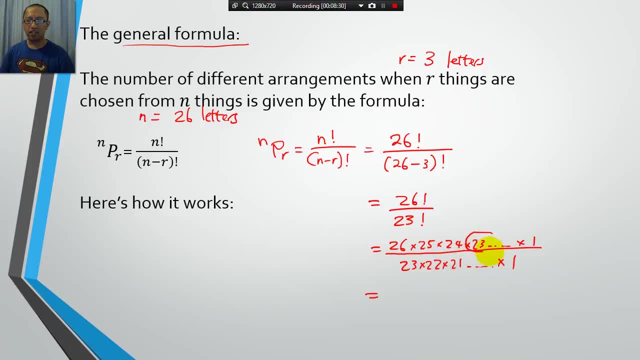 the bottom of the fraction has 23 times 22, all the way down to times 1.. These two numbers are the same, And when the same number divides by itself, you can cross them out and change it to 1, because any number divided by itself is 1.. So therefore, the answer is the same. 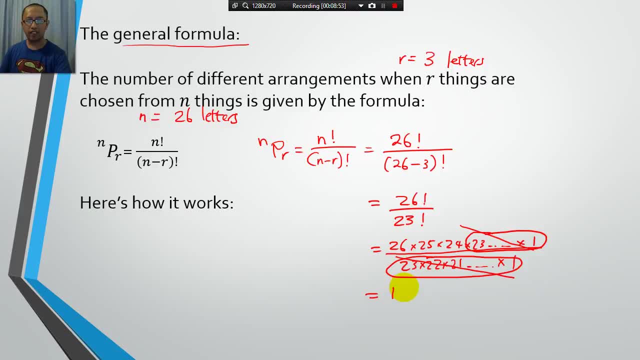 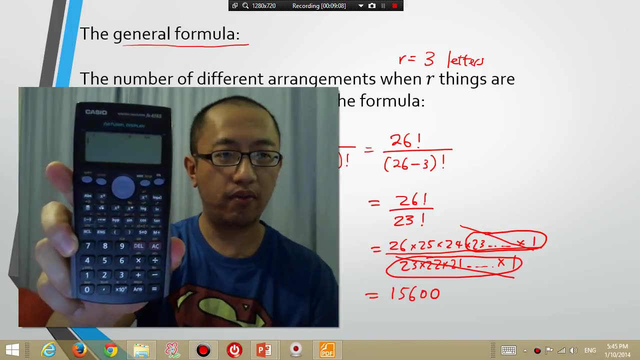 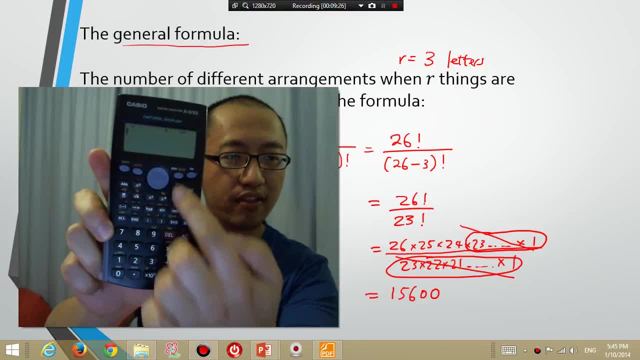 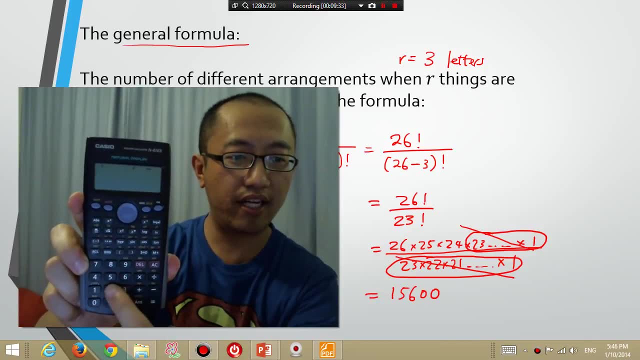 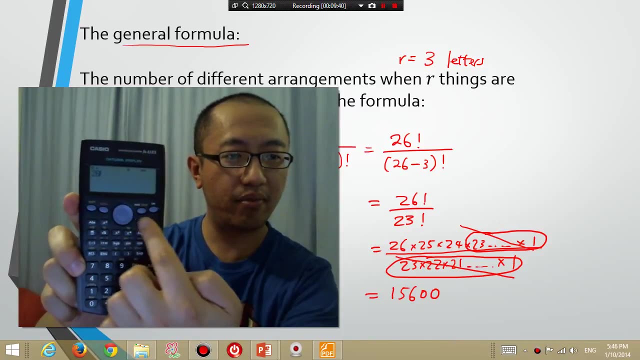 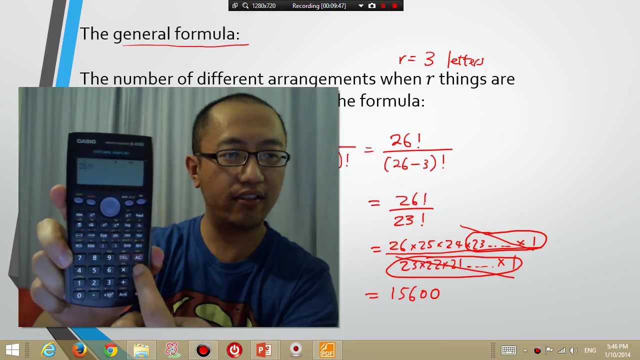 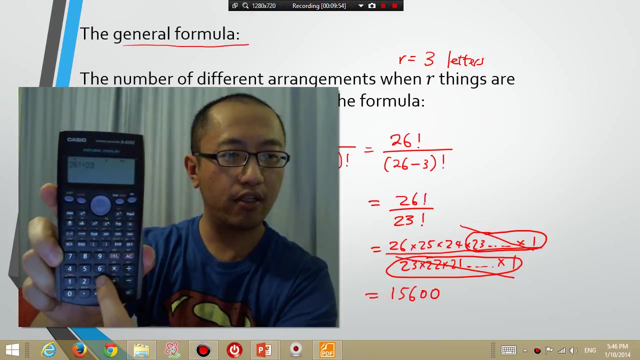 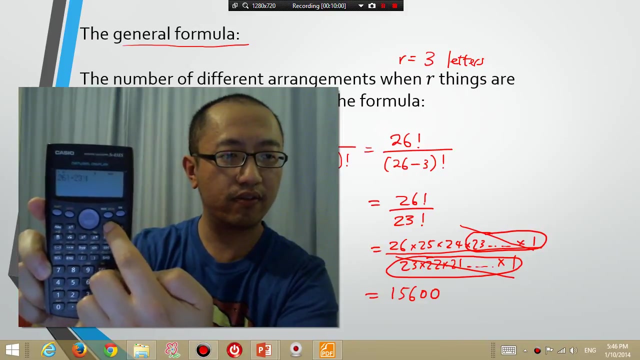 x. this is where the factorial button is. so if you press on the calculator, if you press on the calculator 26, and then press the shift key, and then press the factorial button, and then you press divide, which is this one here divided by 23, so it's kind of hard watching this- 23, and then the shift key, factorial and 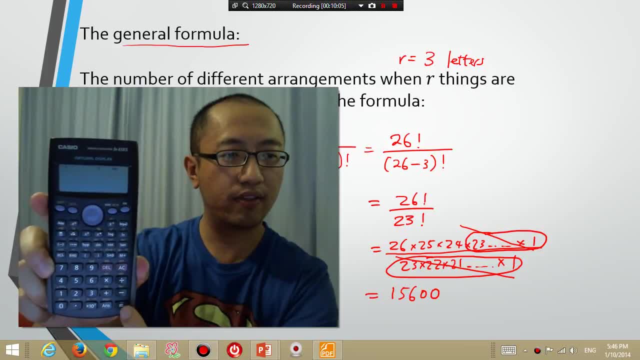 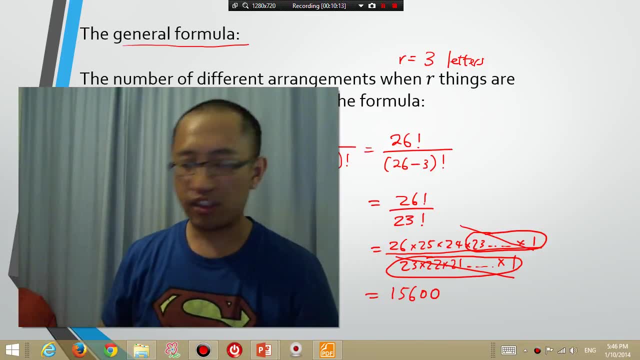 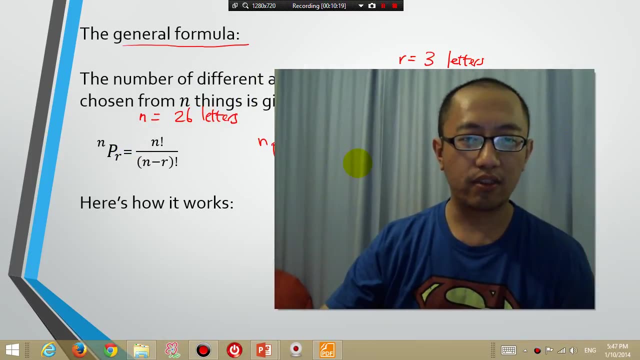 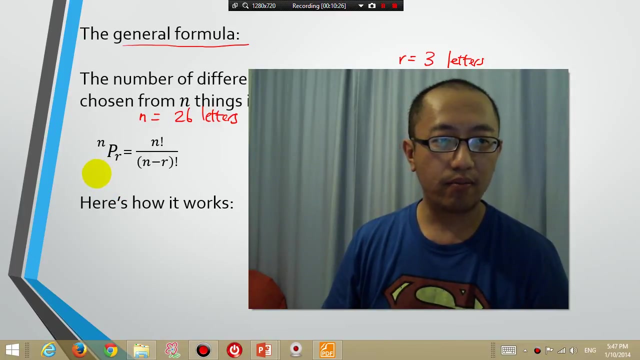 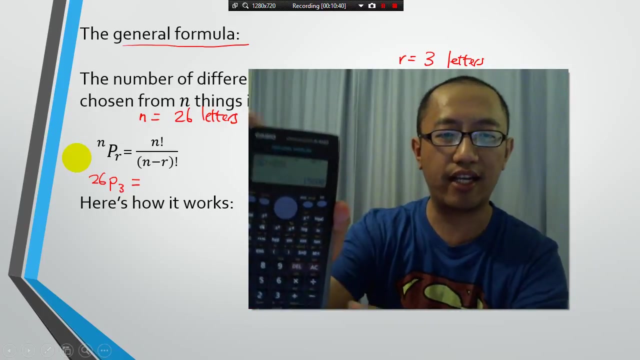 then you press equals, it gives you 15600. but the easiest thing to do is just use the formula NPR, NPR. so actually let me just write it out again. so NPR, here we want 26 P 3. okay, cuz n is 26 and R is 3, so 26 P 3. so if you're gonna use, type that in your calculator. 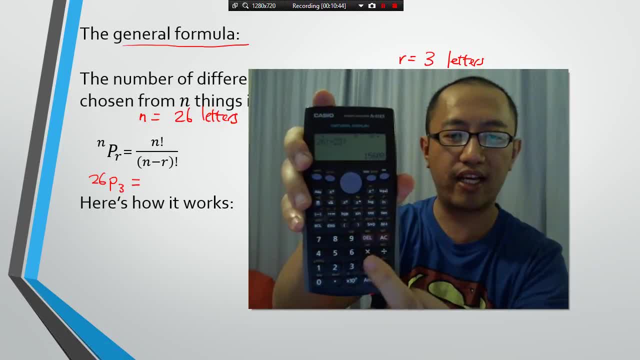 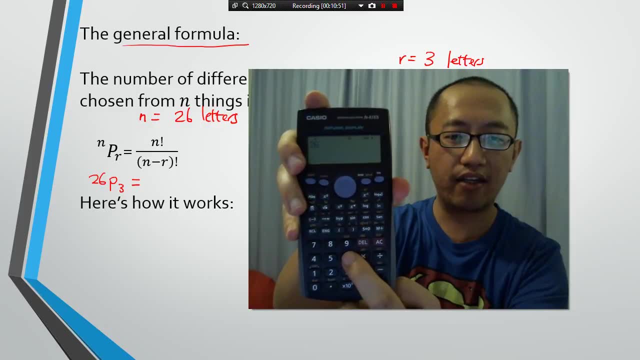 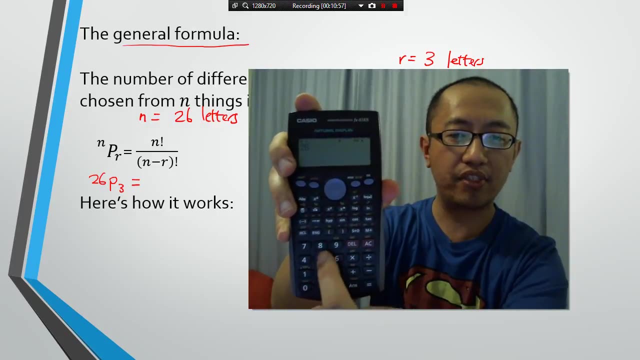 all you're gonna do is put in there 26, where is the P button on your calculator? well, that's actually shift, shift times, and that brings up the P key. and then you can just press 3 and press equals and you get one, five, six, zero, zero. 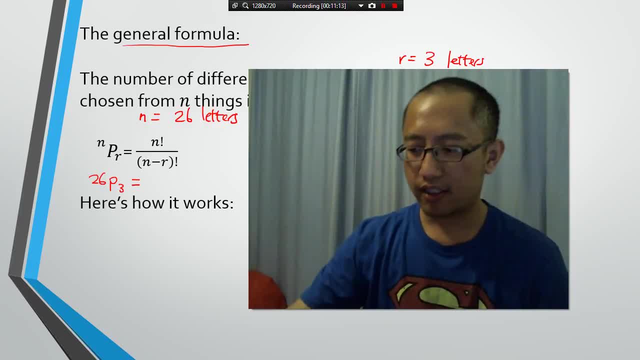 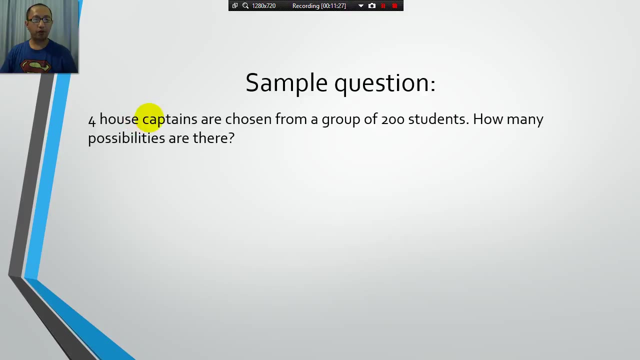 okay, okay, so that's done. okay, do I have a simple problem? so you guys should now find this extremely easy. now, for house captains are chosen from 200 students. how many possibilities are there? well, because the four house captains- each house has a different name. okay, so that's done. okay, do I have a simple problem, so you guys should now.